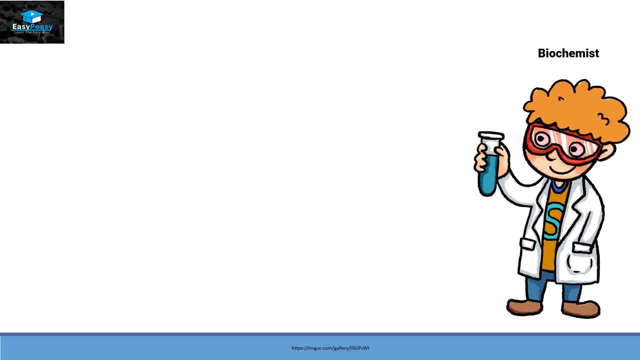 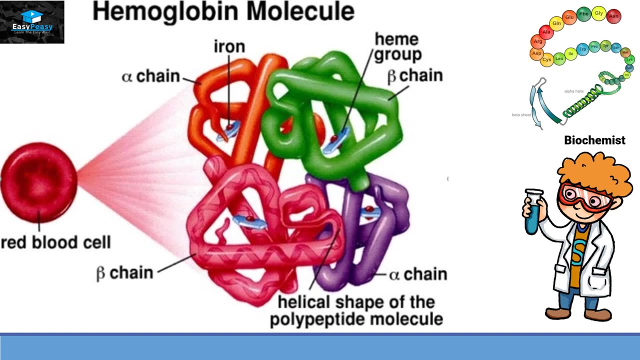 Okay, let's take a biochemist and see how he's going to see things differently than a normal human being. Let's take an example of one macromolecule, and in that case we are going to talk about red blood cells. Now for biochemist. red blood cell is a protein. He will not only be. 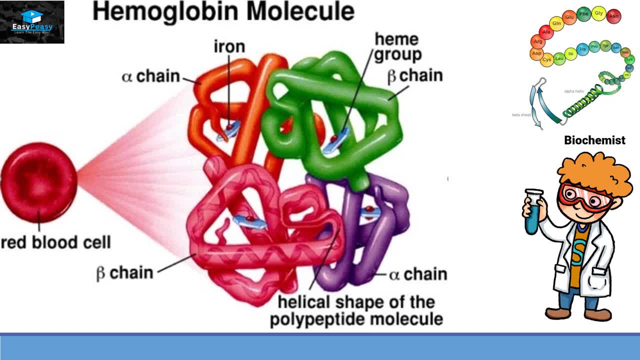 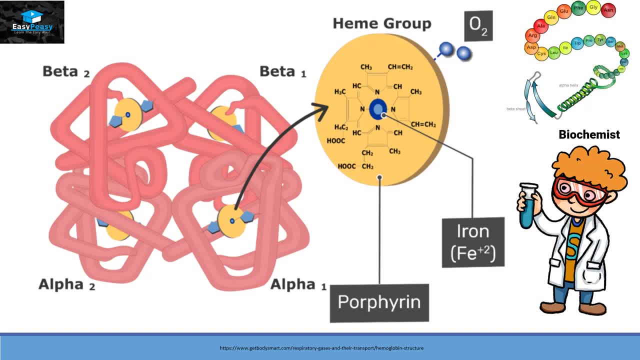 concerned what type of protein is present inside that red blood cell, but he is also concerned with the minute structures present inside this protein. As you can see, this is the heme group, and heme group have iron in the middle surrounded by porphyrin, and this iron is basically involving 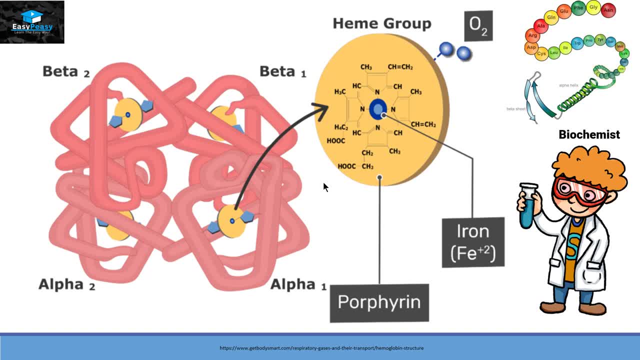 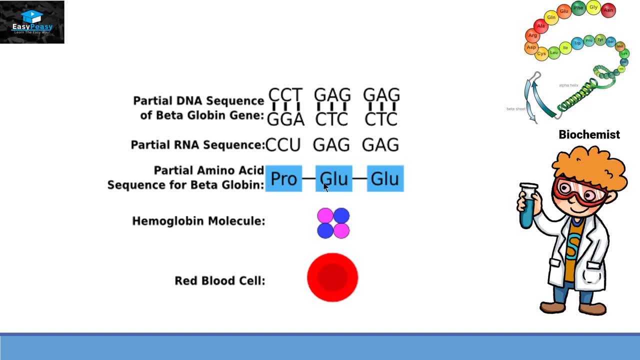 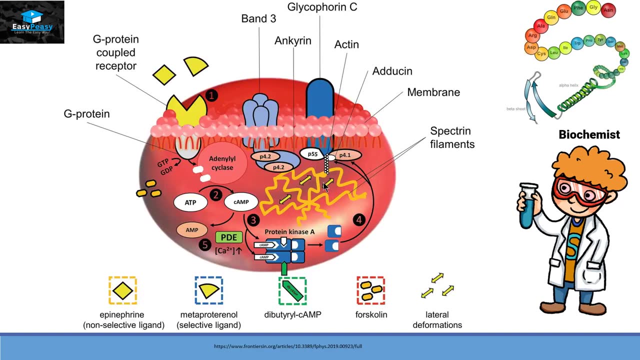 the attachment of oxygen with the red blood cell. Biochemist will also see the sequence of that protein and the DNA that is making this protein. Biochemist will also see what is the function of this protein. Not only the function, but how it is performing this function by using different. 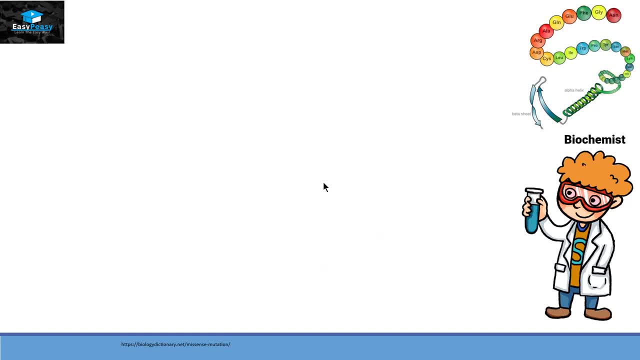 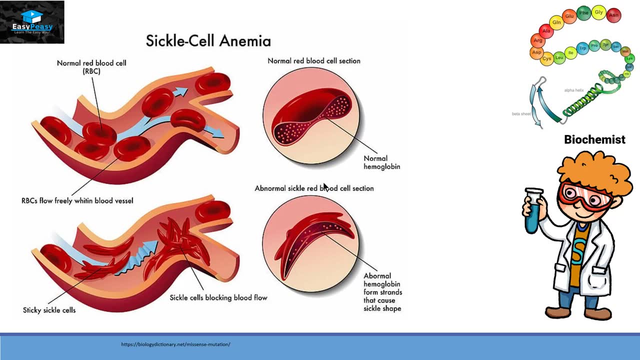 type of enzymes and receptors. Biochemist will also be concerned that if this protein will not work properly, what will happen to that organism? As you can see that if red blood cell doesn't work properly, it will block the veins and that person will be suffering from a disease called. 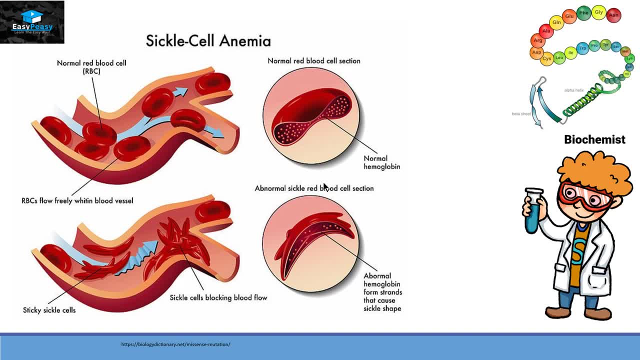 sickle cell anemia. Biochemist will not only be concerned by the function of the protein, but also by the function of the protein. Biochemist will also not only be concerned by the function of the protein, but also by the function of the protein. 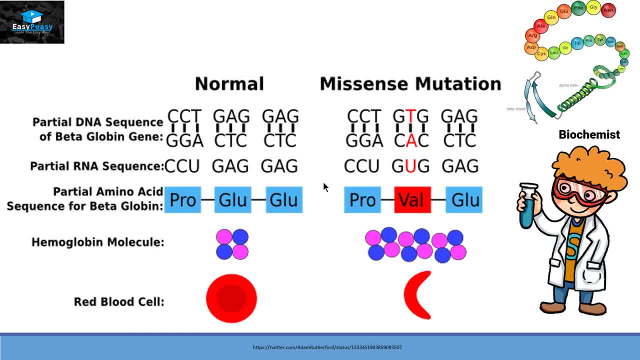 Biochemist will not only be concerned by the effect of this abnormal protein, but he will also identify the mutated genes that are making this protein. As you can see over here, that is, adenine is replaced by thymine, and that's why the glutamine was replaced by valine, and that's why 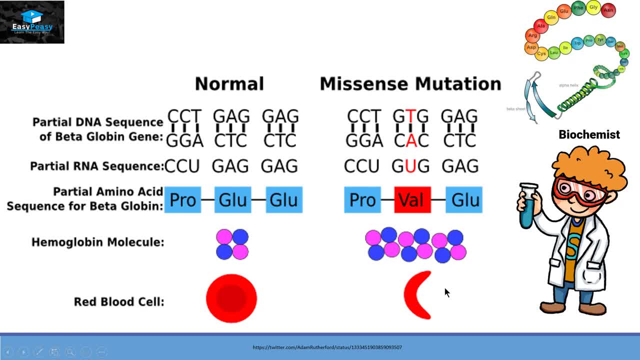 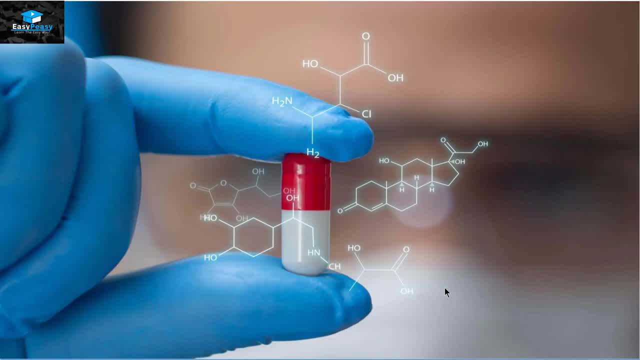 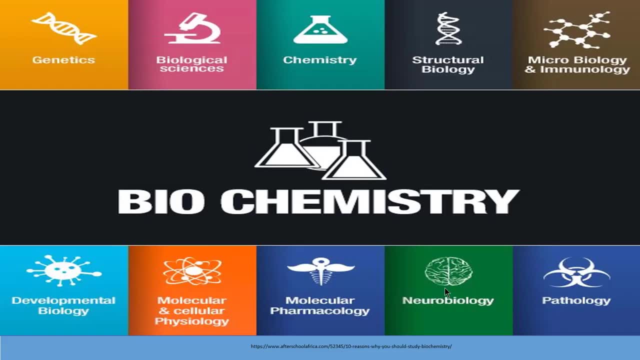 this protein is not made properly and the person is suffering from sickle cell anemia. With all these concepts of looking things deeply inside the organism, this becomes a major step in the pathway of drug discovery. Biochemistry is also concerned with other disciplines. for example, it is: